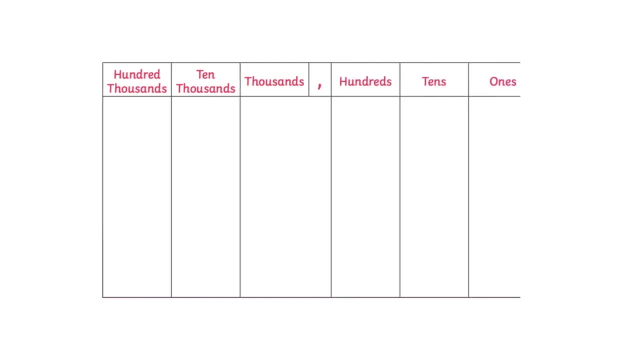 This means, when we are rounding to the nearest tenth, remember to look at the ones digit. If the ones digit is zero, one, two, three or four, then the tens digit stays the same. If the ones digit is five, six, seven, eight or nine, then the tens digit goes up by one. 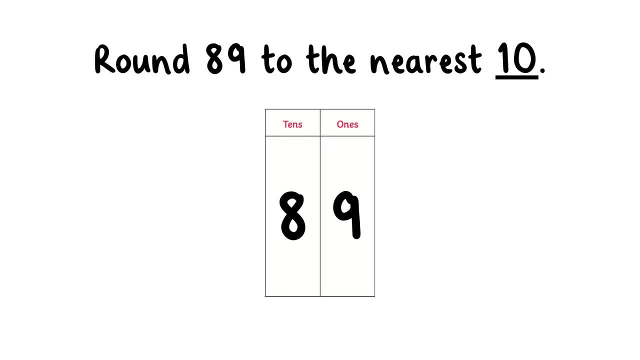 Let's practice Round 89 to the nearest tenth. Since the ones digit is nine, which is five or greater, we increase the tenths digit by one. Therefore, 89 rounded to the nearest tenth would be 90.. Now let's round 574 to the nearest tenth. 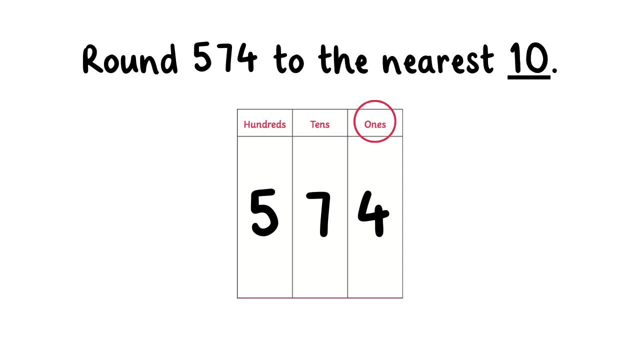 Since the ones digit is four, which is less than five, we keep the tenths digit the same. Therefore, 574 rounded to the nearest tenth would be 570.. Try it yourself: Round 307 to the nearest tenth: 307 rounded to the nearest tenth is 310.. 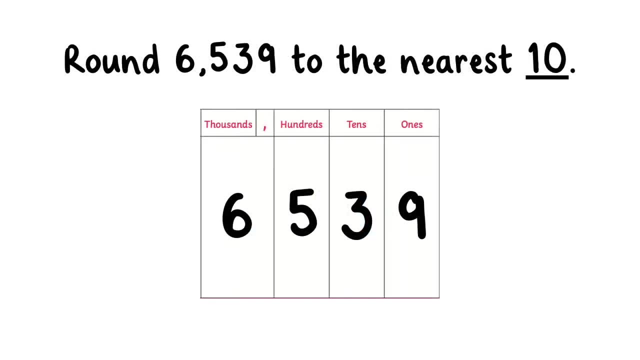 Round 340 and 470 are estimated to be 6.539, which is 6539.. più 1639-a rei Round 936, rounded to the nearest tenth, is 1280.. 6.539 rounded to the nearest tenth is 6.549. 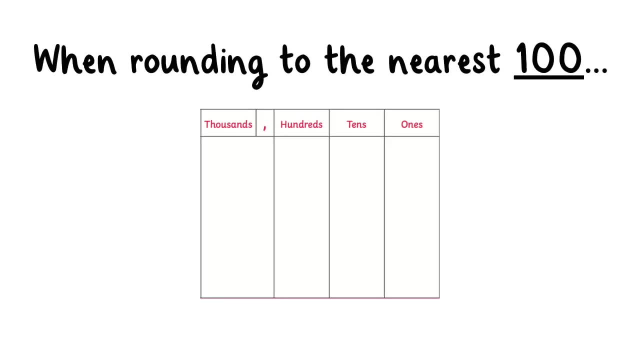 Round 539 rounded to 10 is 530.. 6.539-a- rei Round 6.539 to the nearest tenth is 6.540.. Remember to look at the tens digit. If the tens digit is 0,, 1,, 2,, 3 or 4, then the hundredths digit stays the same.